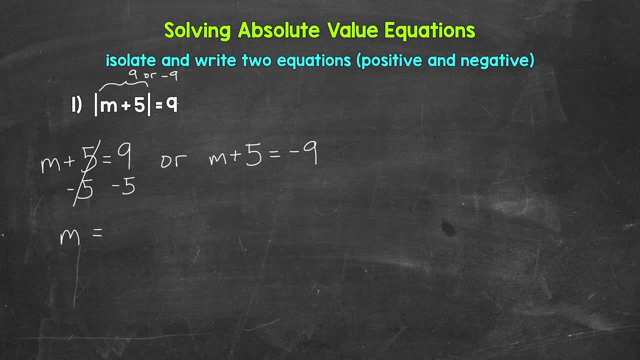 out: m is now isolated, so m equals. and then on the right side, nine minus five gives us four, so m equals four. or let's solve: m plus five equals negative nine now, so we need to isolate m. let's subtract five from the left side. that means we need to subtract five from the right side, as. 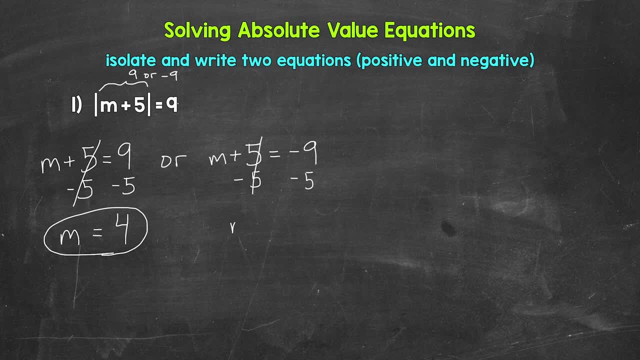 well, these fives cancel each other out. m is now isolated, so we have m equals. and then, on the right side, negative nine minus five gives us negative 14, so m equals negative 14, and those are our two solutions. let's check these solutions by plugging them in for m. so we will start with the absolute. 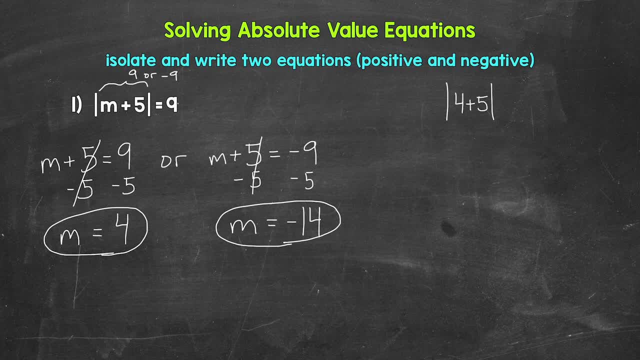 value of four plus five equals nine. and then we have the absolute value of negative: 14 plus five equals nine. let's start with the absolute value of four plus five. well, four plus five gives us nine, and the absolute value of nine is nine. so that is correct. and then, as far as negative- 14 plus five- that gives us: 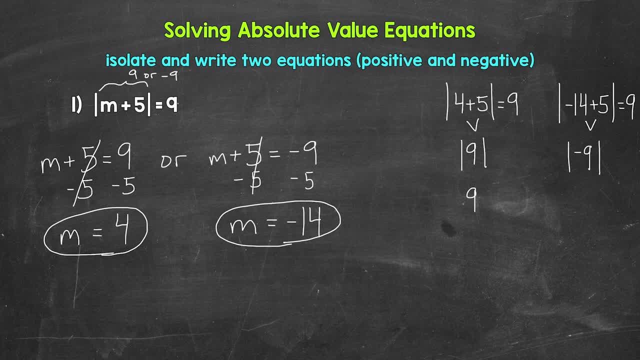 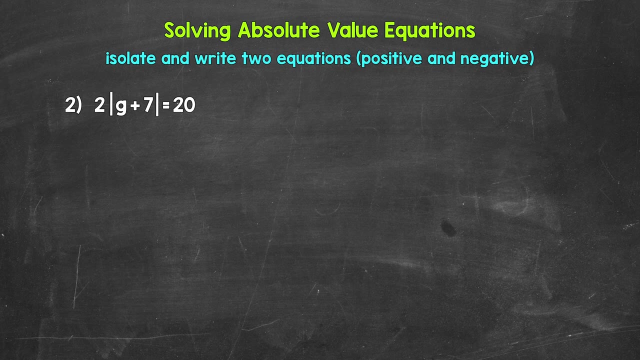 negative nine. so we have the absolute value of negative, and that gives us 9 as well. So we are correct. Those are our two solutions. Let's move on to number two. For number two, we have 2 times the absolute value of g plus 7 equals 20.. Now the 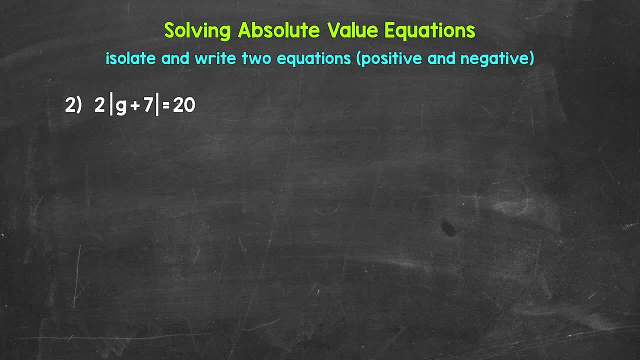 first thing that we need to do when solving an absolute value equation is to isolate the absolute value. So get it by itself. on one side of the equation, We are multiplying the absolute value by 2, so we need to undo that The inverse operation of multiplication is division. So let's divide. 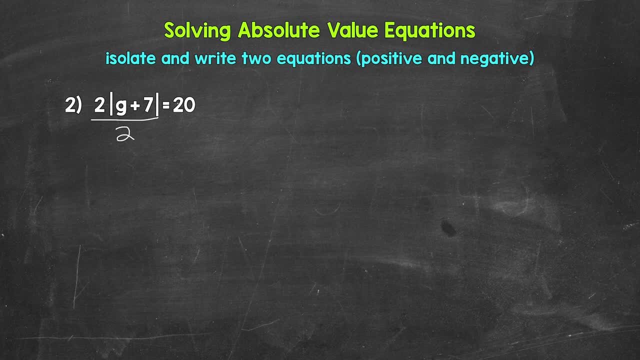 the left side by 2.. Whatever we do to one side of an equation, we must do to the other. So divide the right side by 2 as well. Now, on the left side, these twos cancel usually. So we are correct. Those are our two solutions. Now let's move on to number two. 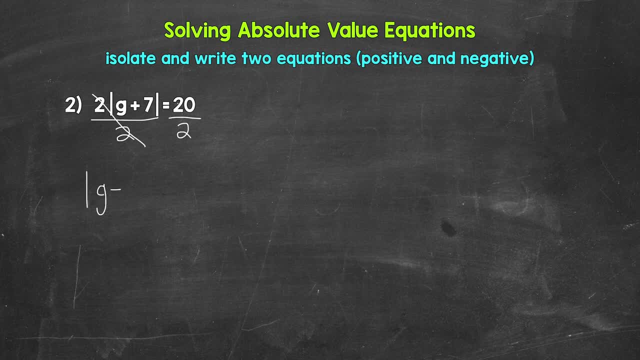 other out. so we have the absolute value of G plus 7 equals. and then, on the right side, 20 divided by 2 gives us 10. so now we have the absolute value of G plus 7 equals 10. the absolute value is now isolated, and now that it is isolated, we 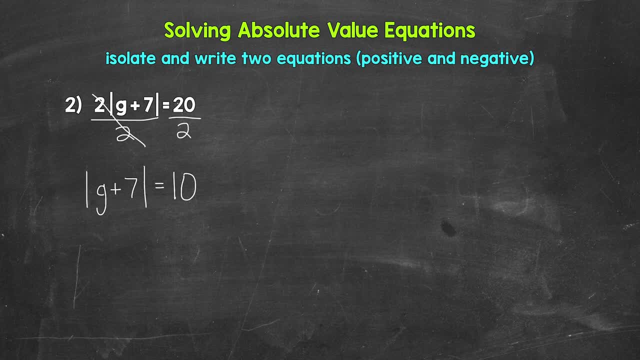 know that the absolute value of G plus 7 has to equal 10. this gives us two options, two solutions. G plus 7 can either equal 10 or negative 10, because the absolute value of 10 is 10 and the absolute value of negative 10 is 10. so 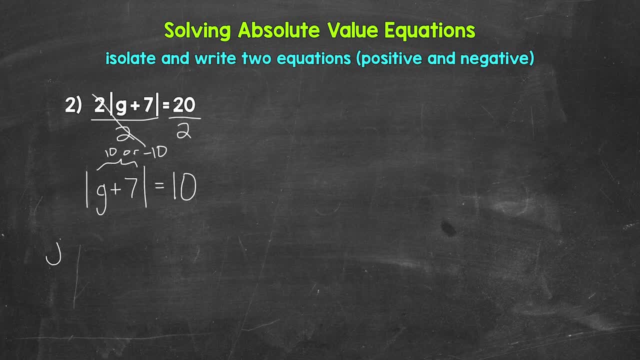 we need to write two equations. we have: G plus 7 equals 10 and the absolute value of negative 10 is 10. so we need to write two equations. we have G plus 7 equals 10, or G plus 7 equals negative 10. now we 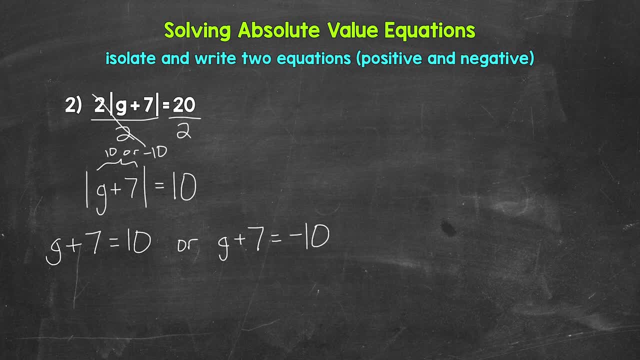 need to solve those to get our solutions. let's start with G plus 7. so let's isolate that variable of G. so we need to subtract 7 from the left side. that means we need to subtract 7 from the right side. these 7s cancel each other out. G is 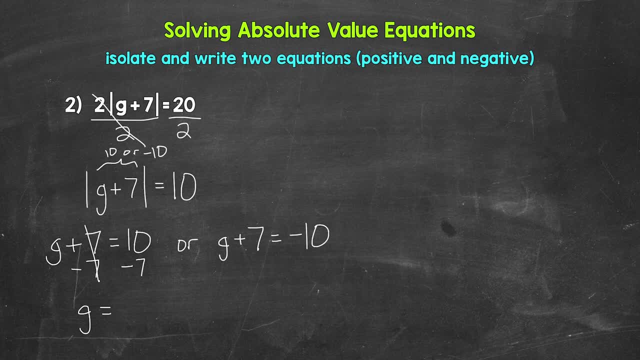 now isolated. so we have G equals. and then on the right side, 10 minus 7 gives us 3, so G equals 3. now let's solve: G plus 7 equals negative 10. so let's subtract 7 from the left side and the right side. these 7s cancel each other. 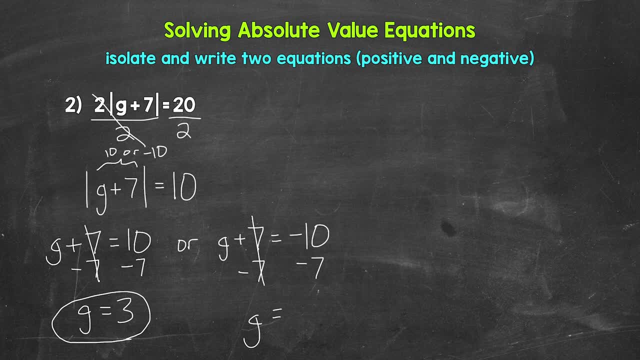 out. so G is now isolated, G equals. and then on the right side, negative 10 is Safety. to be safe, Party out of motion when to find G plus g of zero, 0.這個轮 we can check those solutions by plugging them in for G and seeing if they work. so ag can. come to the side here. so we have two times the absolute value of 3 plus 7 equals 20, and then 2 times the absolute value of 3 plus 7 equals 20, and then two times the absolute of 3 equals 20, and 2 plus 7 equals R1 equals 20, and 2 times the absolute value of 3 plus 7 equals R1 equals 70, and then 2 times the absolute value of 3 and 2 times the absolute value of 3 equals R1 equals R1, equals. clearly explain all these features and this is what we considered. If you are not familiar, we will be looking at where the answer is. if you have any questions and if you need help, especially if you would like to correct me, please answer what the answer is. 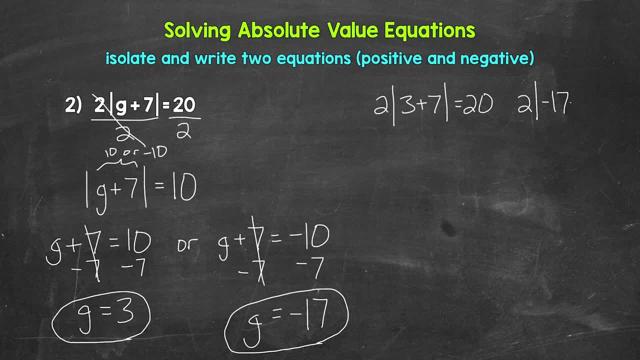 absolute value of negative. 17 plus 7 equals 20.. And let's start with 2 times the absolute value of 3 plus 7.. 3 plus 7 is 10.. So we have 2 times the absolute value of 10.. The absolute value of 10. 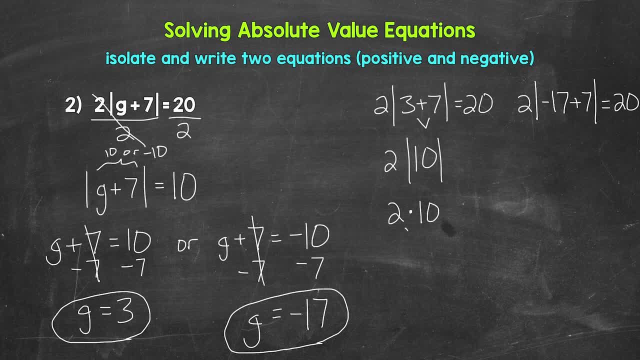 is 10.. So now we have 2 times 10,, which is 20.. So we are correct there. G equals 3.. Let's do 2 times the absolute value of negative 17 plus 7. now Let's start with negative 17 plus 7.. That gives: 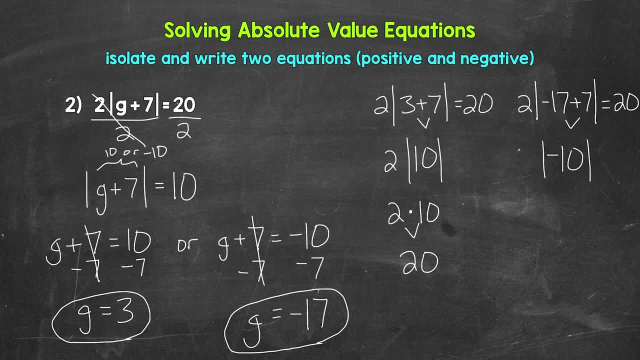 us negative 10.. So now we have 2 times the absolute value of negative 10.. The absolute value of negative 10 is 10.. So now we have 2 times 10.. 2 times 10 is 20.. So we are correct there as well. G equals negative 17.. 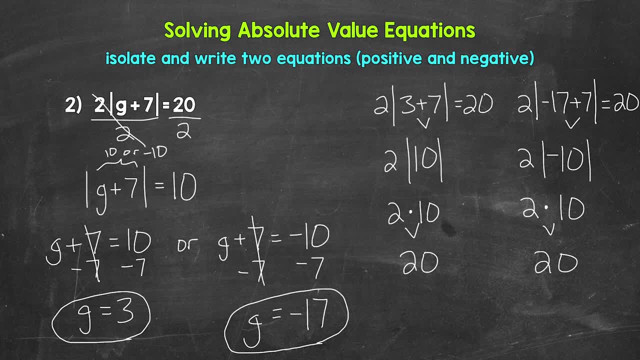 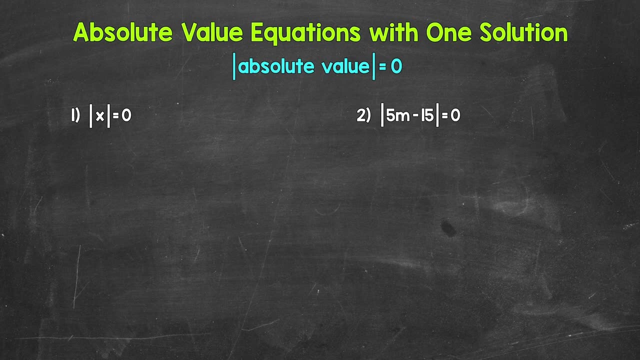 So again, our two solutions here for this example 3 and negative 17.. So there's our two solution section. Let's move on to some examples with one solution. Here's our section on absolute value equations with one solution. Let's start with the absolute value of negative 17 plus 7.. The absolute value of negative 17 plus 7. 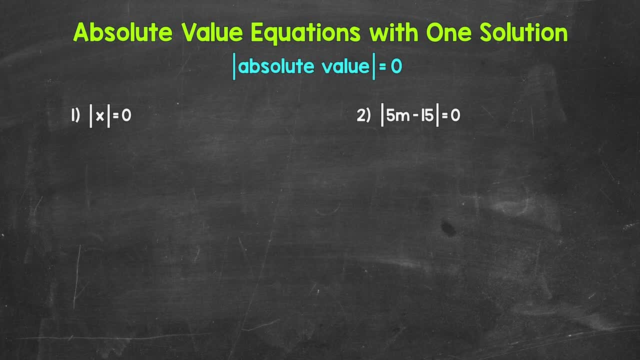 is 0.. Let's jump into number 1, where we have the absolute value of x equals 0. Now remember, the absolute value of a number is its distance from 0. So what does x have to equal here? Well, 0. There's only one possibility, one solution: x equals 0. And that's our one solution. 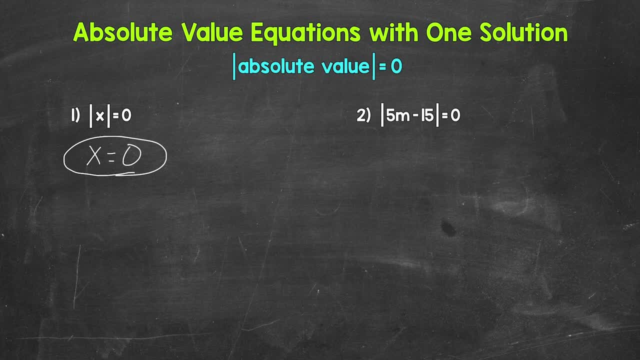 So let's compare that to another example. here Let's say we have the absolute value of y equals 7.. Now here we have two possibilities, two solutions. Y can equal 7. Or y can equal negative 7.. The absolute value of 7 is 7, 0. And the absolute value of negative 7 is 7.. So y equals 7. Or y equals 3.. 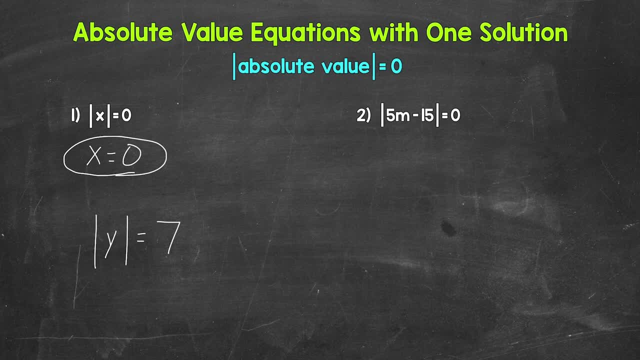 So here we use a new would-be kg model to compare. to put it that way: Get the y-axis for y equals 1, and the y-axis for y is 2.. x is equal to negative 8.. There's no problem with that, all right. 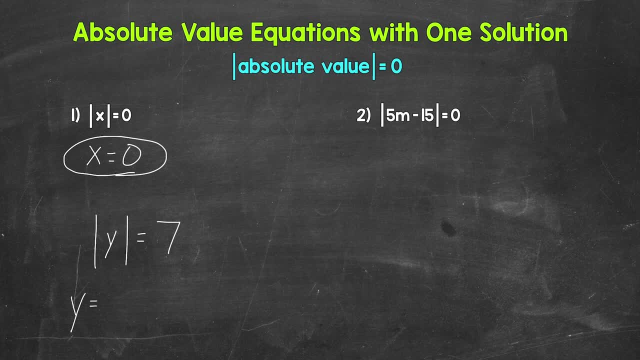 Again, this will have some more вариантs to round it all out, but it's just a reason for everybody to reflect on the constant. So we want to get this. so we're going to come into the large or even ев and togehen to curve this formula into a fairer version here, Which is, if y equals 7 – x is equal 7.. While, because this guy'sassa. 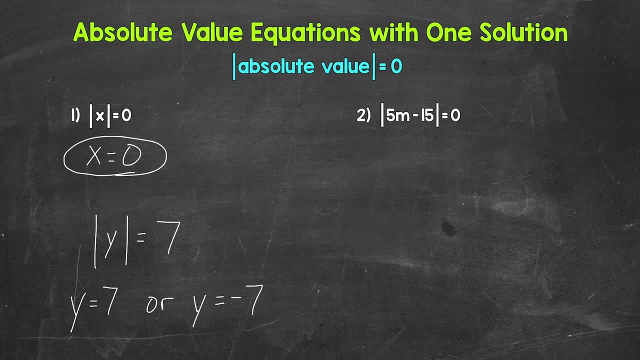 y equals negative 7.. We have two solutions. So keep in mind, when we have the absolute value of something and it equals 0, we have one solution, because whatever is inside of the absolute value has to equal 0.. Let's move on to number 2 and take a look at another example. 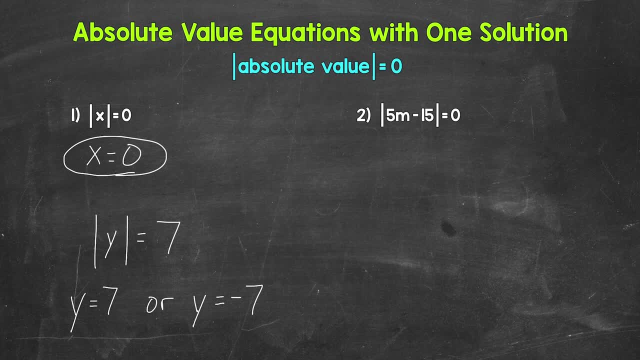 We have: the absolute value of 5m minus 15 equals 0.. Now here we know that 5m minus 15 has to equal 0, because the only possibility to make this work is 0.. The absolute value of 0 equals 0.. 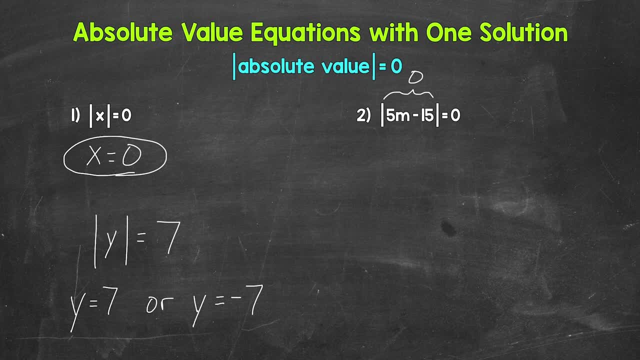 So, in order to find the solution, we need to solve: 5m minus 15 equals 0. And this will give us one solution In other situations. we have to write and solve two equations, One equal to a positive and one equal to a negative. 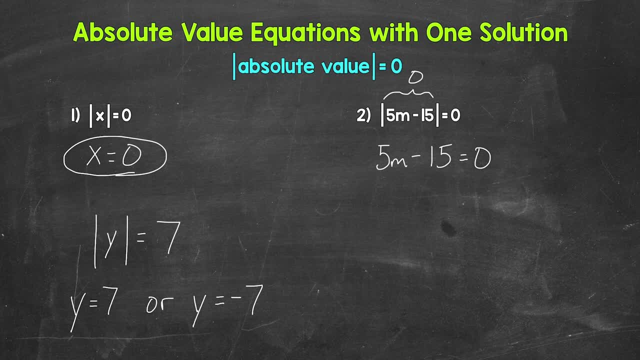 But here we only have one option, 0. So now we need to solve. So let's isolate m. We need to undo the subtraction first, So let's add 15 to the left side of the equation. That means we need to add 15 to the right side as well. 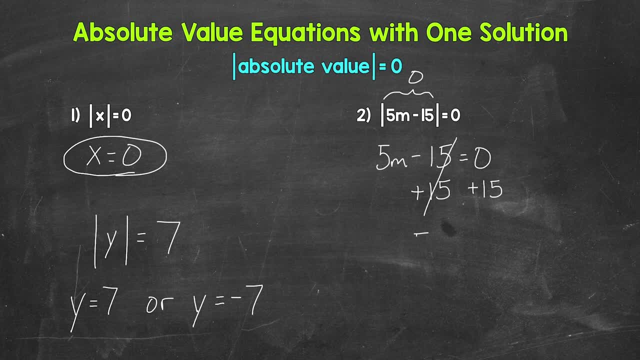 The 15s on the left side cancel each other out, So we have 5m equals. On the right side, 0 plus 15 gives us 15. So we have 5m equals 15.. Let's divide the left side of the equation by 5. 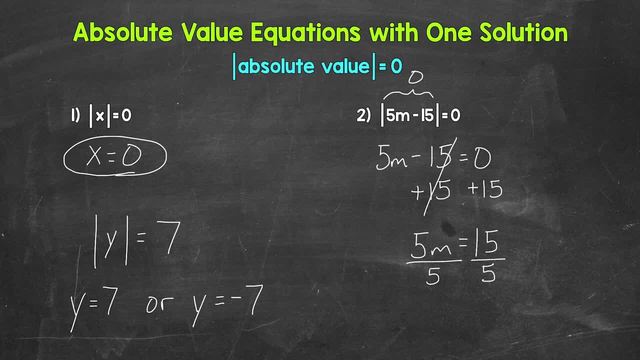 and divide the right side by 5 as well. These 5s cancel each other out, So m is now isolated. And then on the right side, 15 divided by 5 gives us 3. So m equals 3.. That's our solution. 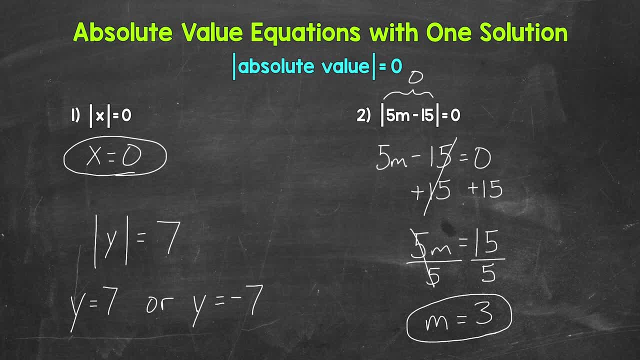 Our one solution, And we can check this solution by plugging it in for m. So let's come to the side. here We have the absolute value of 5 times 3 minus 15 equals 0. So 5 times 3 gives us 15.. 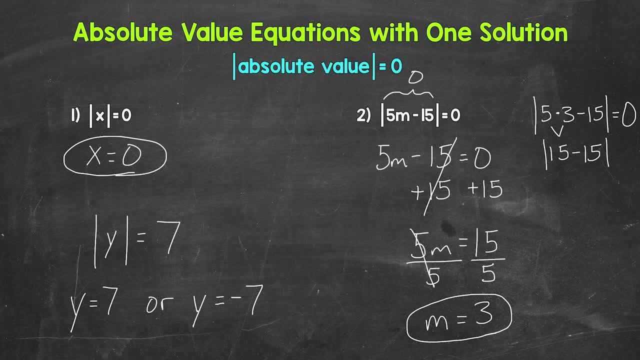 So now we have the absolute value of 15 minus 15.. 15 minus 15 is 0. And the absolute value of 15 minus 15 is 0. And the absolute value of 0 is 0. So we are correct. 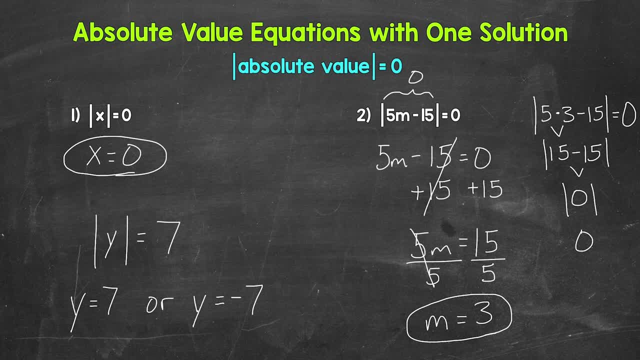 m equals 3.. So there you have it. There are a couple of examples of absolute value equations with one solution. Just remember, if you have an equation where the absolute value is equal to 0,, you'll have one solution, And this is the case whether the absolute value equation is already isolated and equal to 0,. 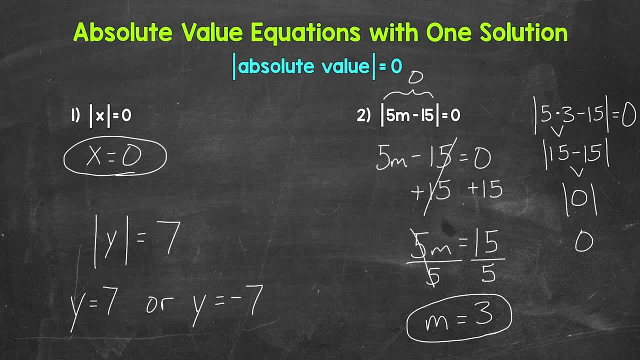 like these examples, Or if you need to solve a problem, you can do that. But if you need to isolate the absolute value first, and then it ends up being equal to 0, you'll have one solution for that as well. So there is our one solution section. 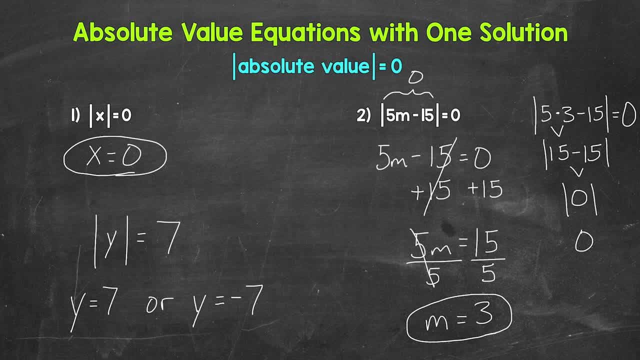 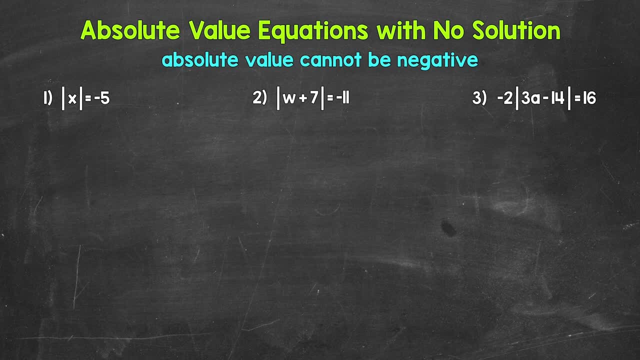 Let's move on to absolute value equations with no solution. Let's take a look at absolute value equations with no solution. Now keep in mind: the absolute value of something, whether it's a number or an expression, cannot be negative. It cannot equal a negative. 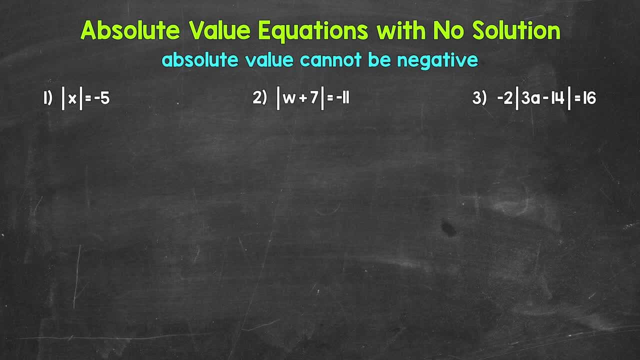 The absolute value of something is always going to be positive or 0. So keep that in mind. Let's jump into number one, where we have: the absolute value of x equals negative 5. Now again, and this is very important- the absolute value of something cannot be negative. 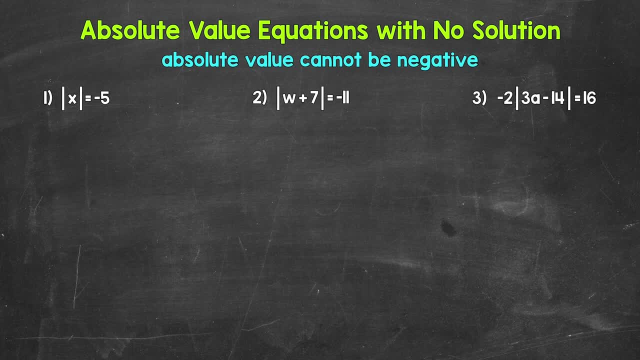 There's no way to make this work here. There isn't anything x can equal and the absolute value will equal negative 5.. Now you may be thinking: how about negative 5?? Well, the absolute value of negative 5 is 5, so that won't work. 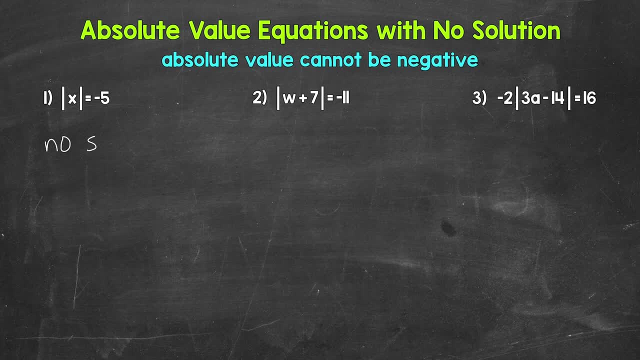 There is no solution for this equation. Let's move on to number two and take a look at another example. We have the absolute value of w plus 7 equals negative 11.. So, again for this one, we have the absolute value and it equals a negative 5..